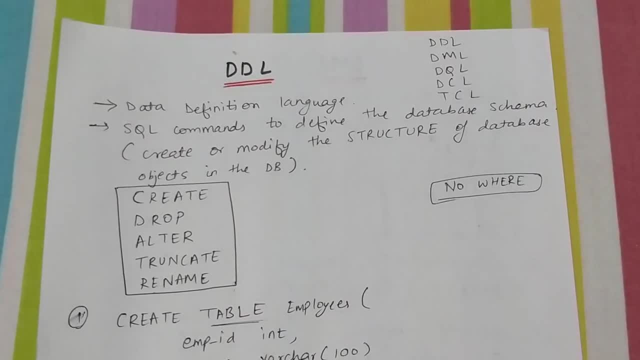 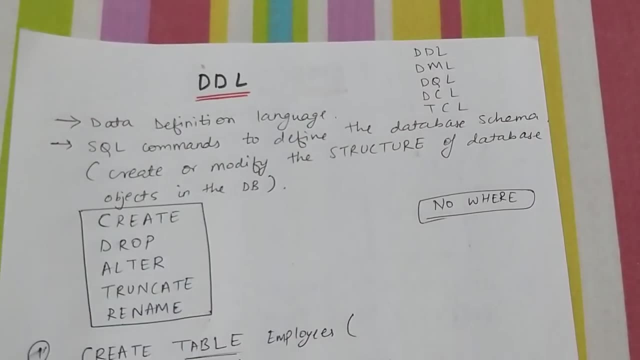 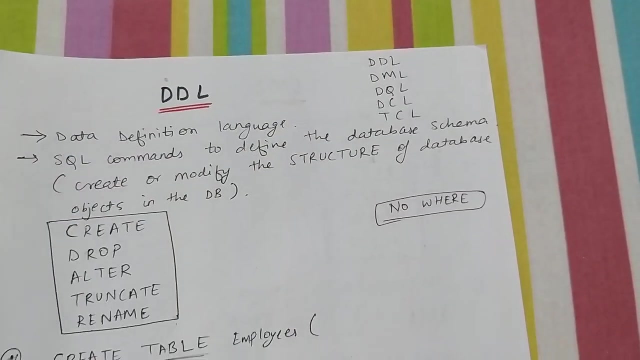 Hello everyone, welcome back to my another video. So in this video we are going to study about DDL. So what is DDL? DDL is Data Definition Language And similarly there are other commands also like DDL, DML, DQL, DCL, DCL, and those videos will come soon. 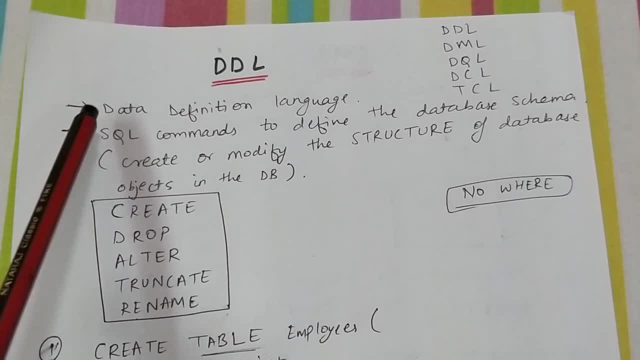 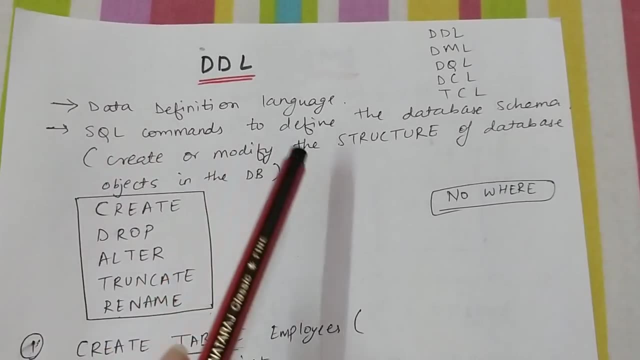 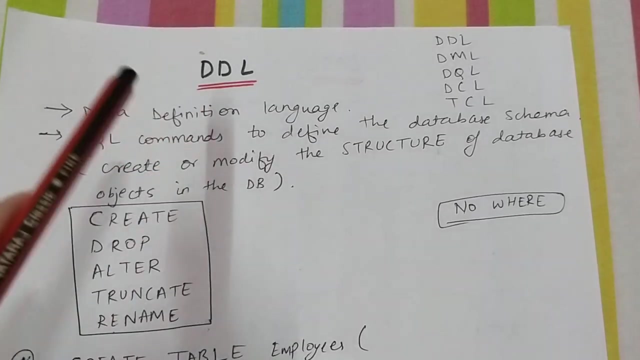 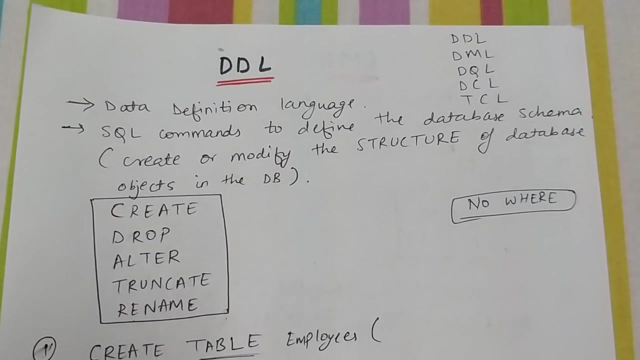 So what does data definition language mean? So basically, DDL is what SQL command? Those are commands to define the database schema. So basically, you are going to define, because data definition language so hence define. So hence these commands will define the database schema, Database schema as in tables and all. So we are basically going to create tables or drop tables or alter. Basically we are going to define. 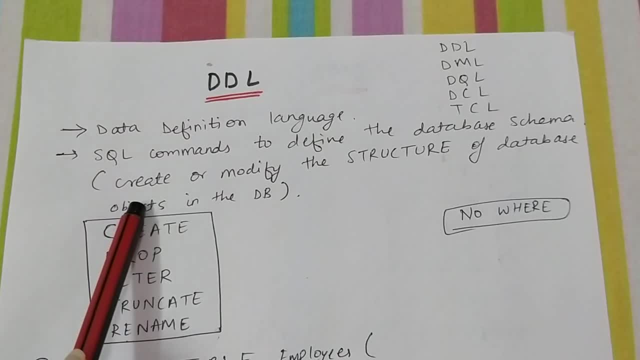 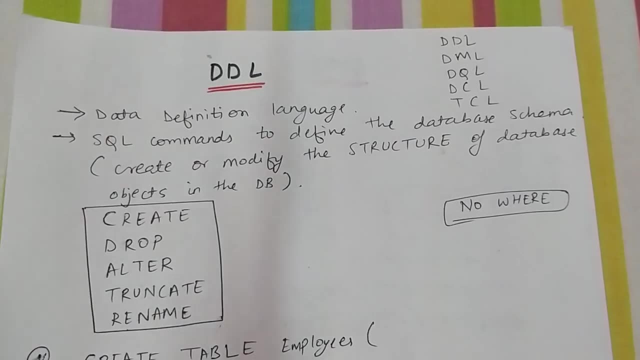 Those structures, database schemas. So basically you will create or modify the structure of database objects in the DB, And database objects means tables, views and all of that. So basically we are going to create them or modify them. the structure of database objects. 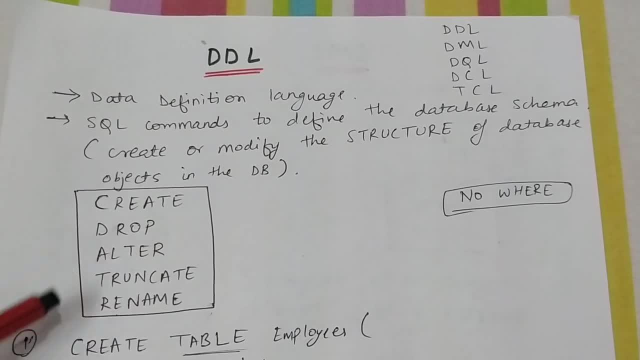 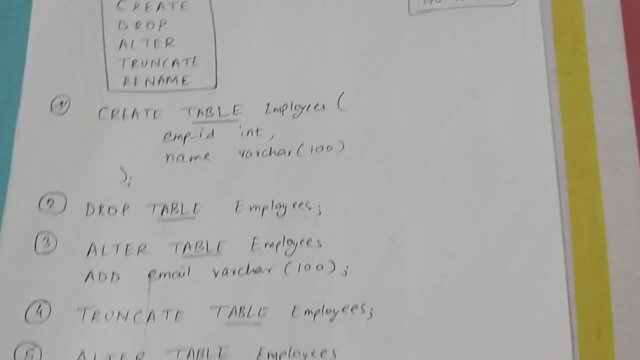 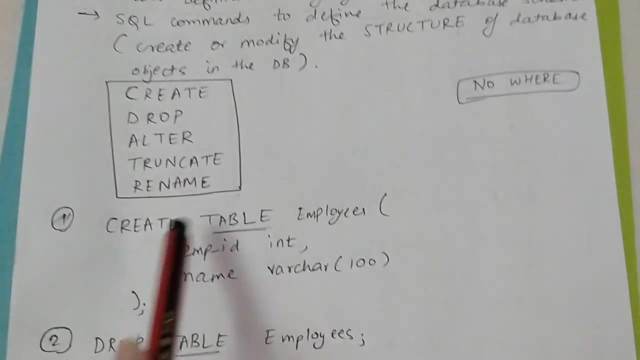 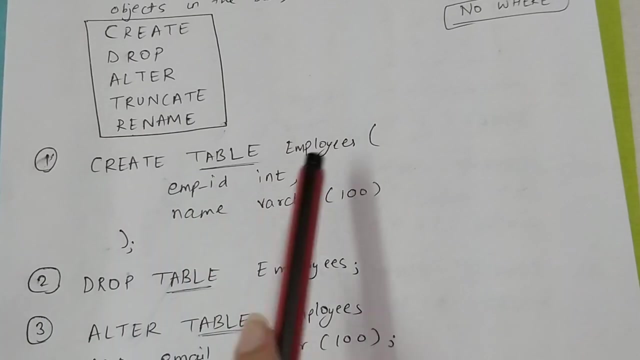 So there are five DDL commands. So those are: create, drop, alter, truncate, rename. Let's see one by one. Okay, so the first command is create. So the first one is create. So we are creating a table, We are creating a DB object. So we are creating a table, Create table, employees and whatever columns you want to add: Employee ID, name and their data type. So this is how we are creating a table. 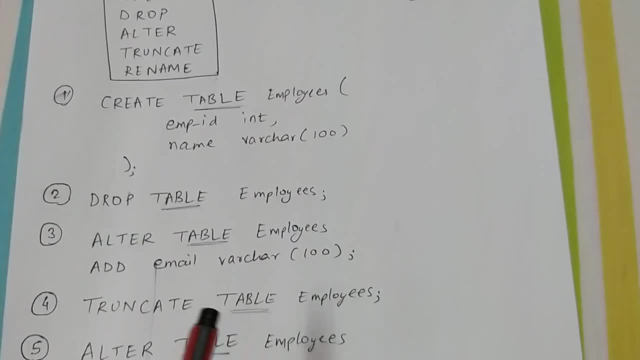 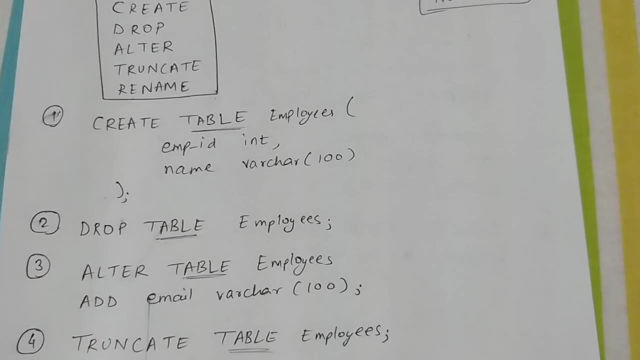 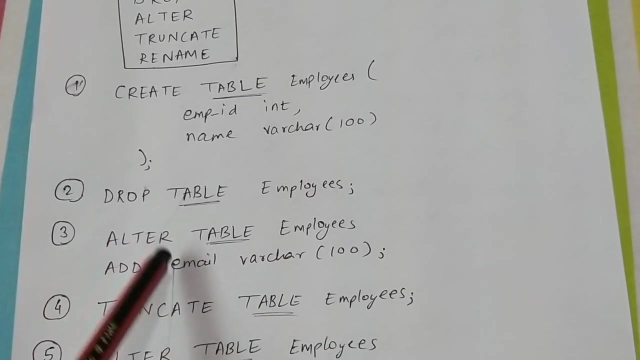 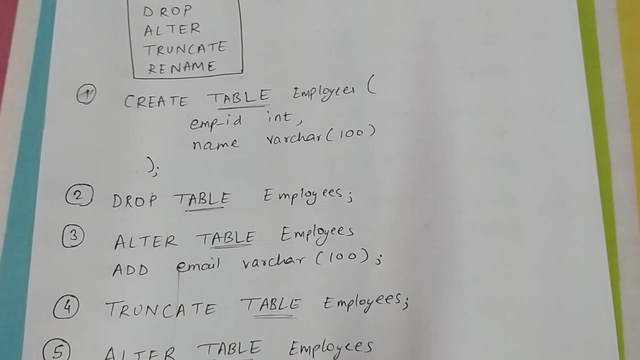 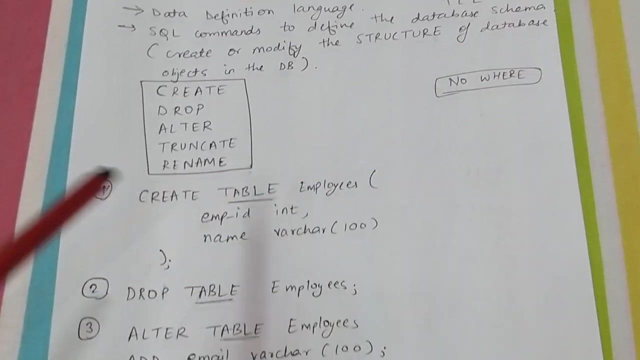 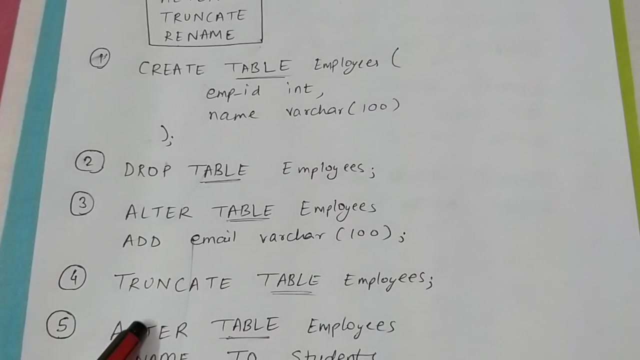 Then if you want to drop the table, then we have drop table employees. Then if you want to alter the table, if you want to add an, add an column, sorry, add a column to the table. So if you want to add a column or if you want to, you know, change the data type of a particular column, So basically you're going to alter the table because you are changing the columns, columns in the table. So basically you are changing the structure of the database. Okay, so basically you're defining it again. So that is alter. Then we have truncate table employees. So what does truncate do? 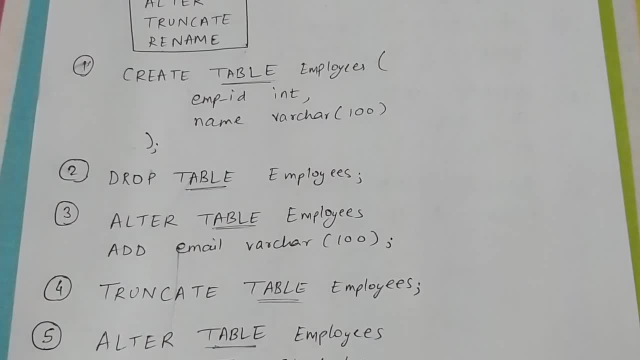 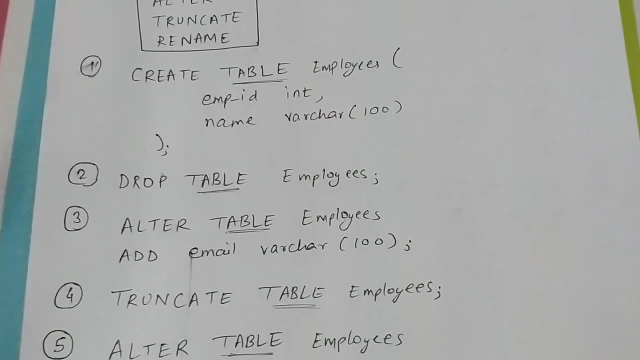 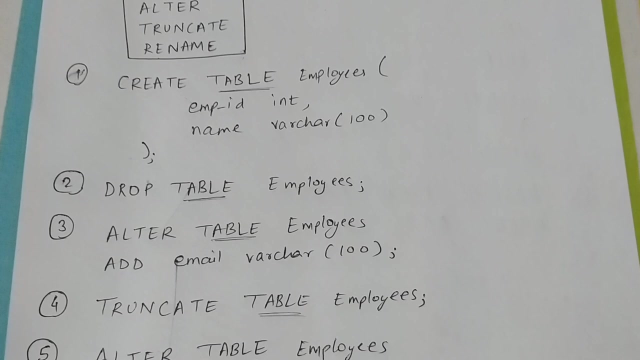 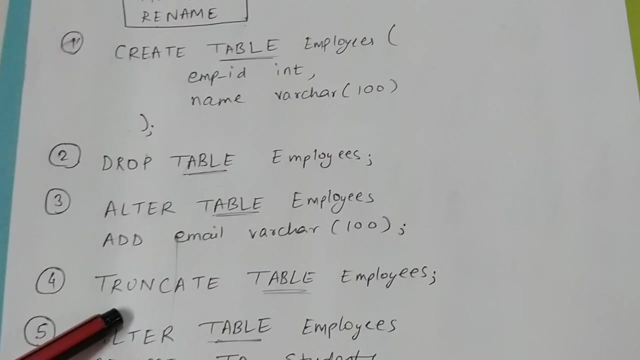 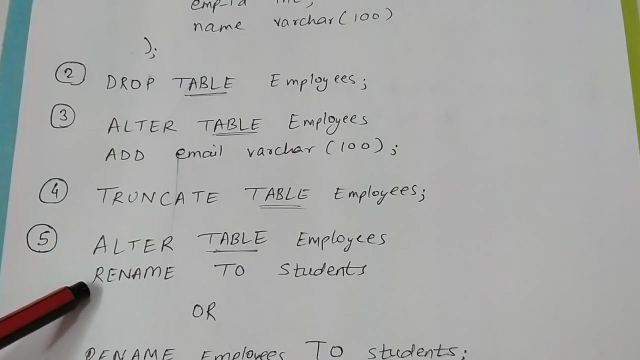 So truncate will remove all the All the rows. Now you will ask me: how is truncate a DDL? because it is not defining the structure, It is just removing the rows. No, it is not just removing the rows, It is deallocating the space allocated to those rows And hence, hence, it is changing the storage definition. So here it is changing the storage definition. Okay, in case of truncate. Okay, in case of truncate, it is changing the storage definition. Hence, it is in DDL. Okay, and our fifth command is alter. 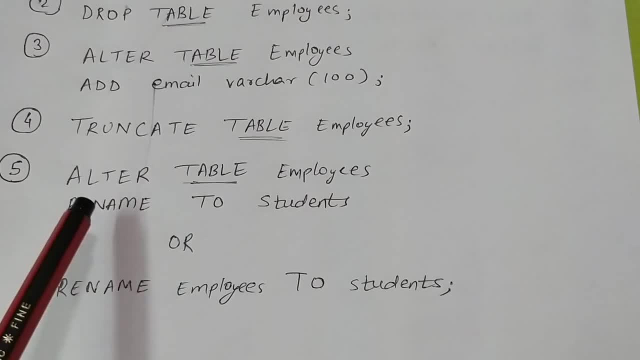 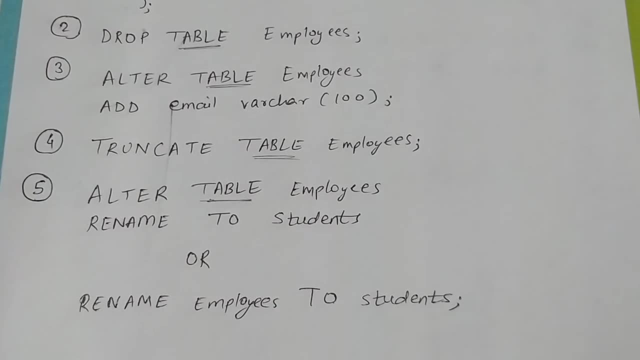 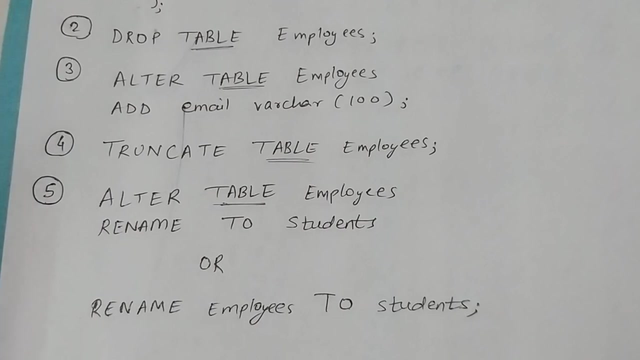 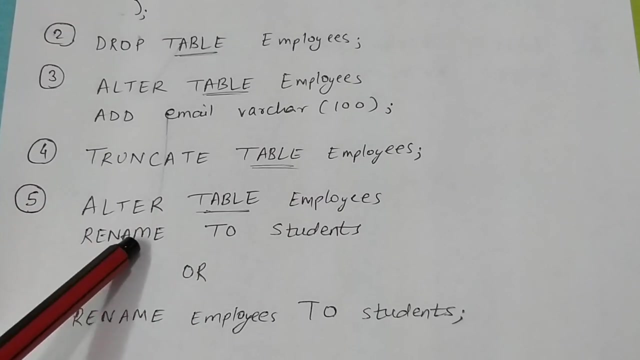 Rename, As I said, rename. So what is the command for rename? Alter table employees, whatever the name of the table is Rename to students. So I'm changing the table name from employees to students. Hence we are redefining it and redefining the name of the table and hence it is a DDL command. So basically, there are two ways how you can write a rename, Rename command. So one is this one and the other is simply write rename employees to students. So there are certain things which you can do. 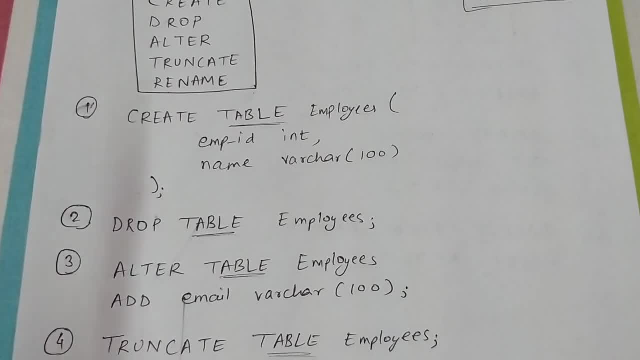 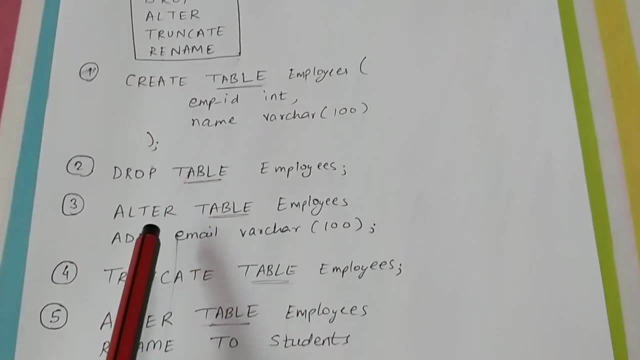 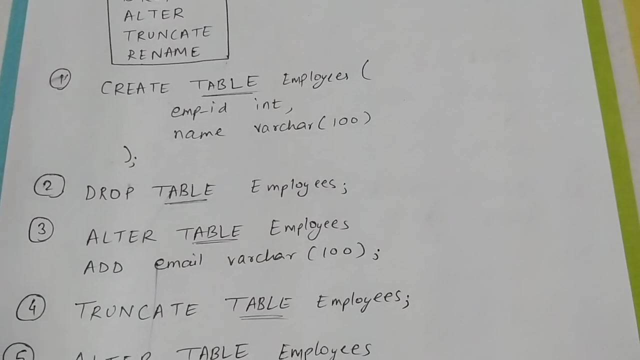 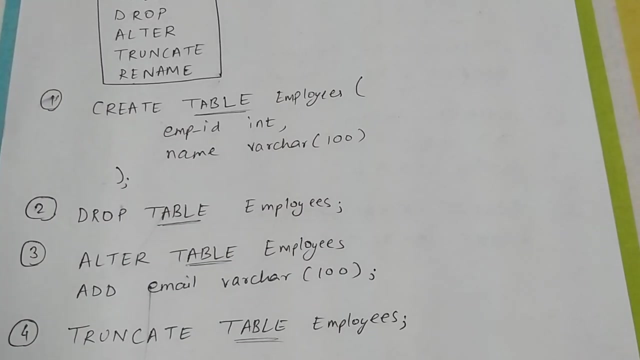 You should remember or should keep at the back of your mind. So one thing is: in DDL commands you will always have the word table in it. So create table, drop table, alter table, truncate table, alter table. So and in case of DML or any other like insert queries or delete queries or something there, we do not write the word table. Okay. so in this case, as we are defining a structure, so we write. sorry, we're defining the structure of a database object, So we write. 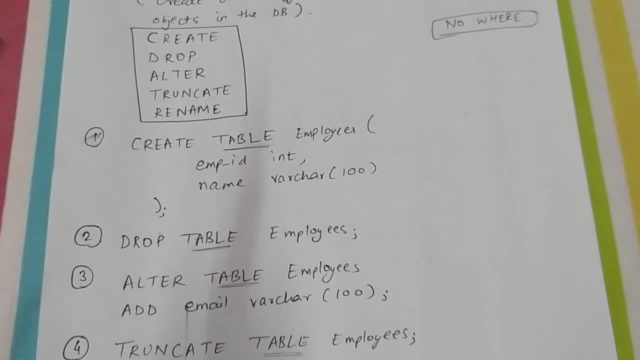 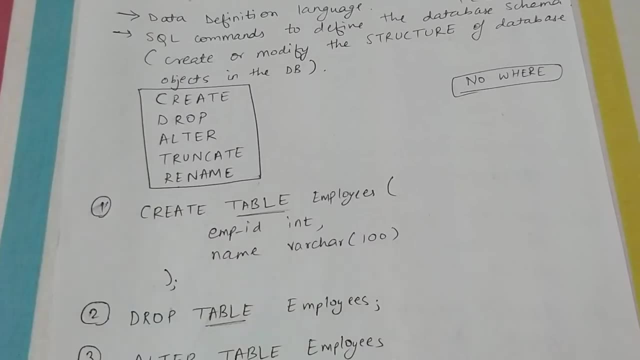 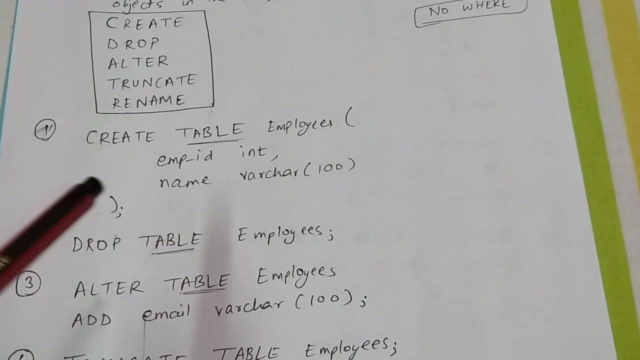 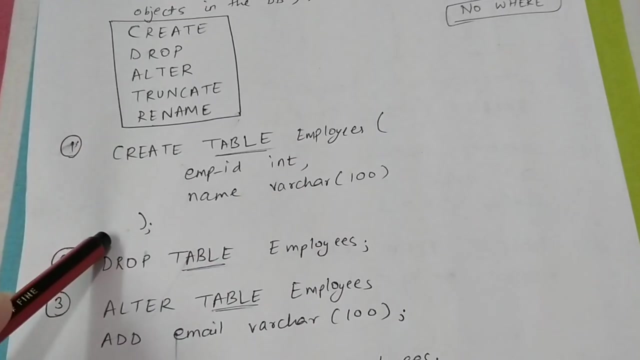 the object name, like create table, drop table and all Also. one more thing we need to keep in our mind is there is no where in these commands- Okay, so you all must have seen the query for insert, insert or update. We always write where: Update this, this. this set this to this where something is going to something. But in data definition we do not use where in it. So this is DML. 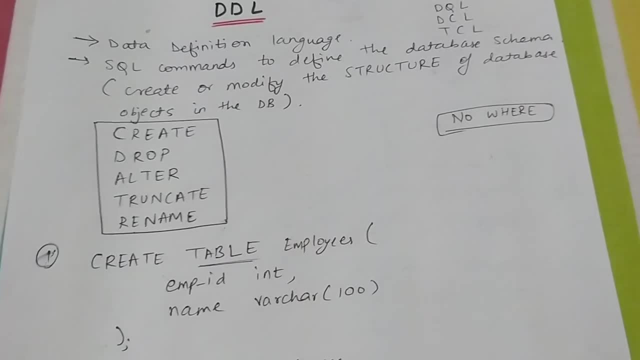 I hope it was clear, And these videos are coming soon, So do subscribe to the channel. Thank you for watching.